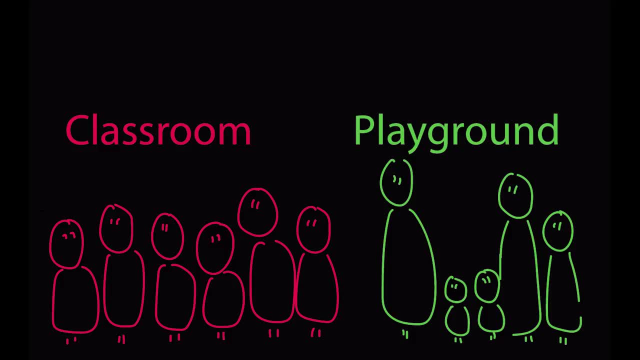 the two groups differ in relation to height. So let's start looking at the average height of the people in each group. In the classroom, the average height of the students is this line here. So what this white jagged line represents is the average height of the students In the playground. 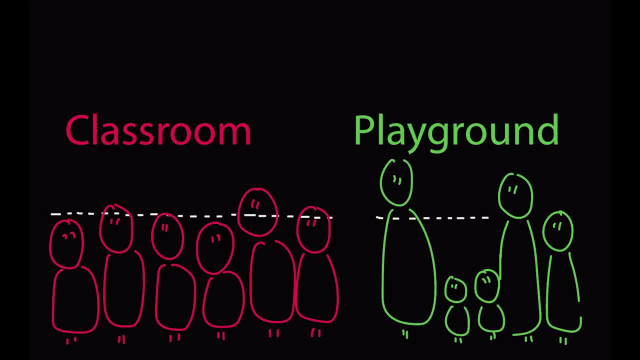 the average height of the mommies, the daddies, the babies, the toddlers is, as it turns out, the exact same as the average height of the people in the classroom. So, if we're to go back and think about our question, how do the two groups differ in relation to height? it's not because 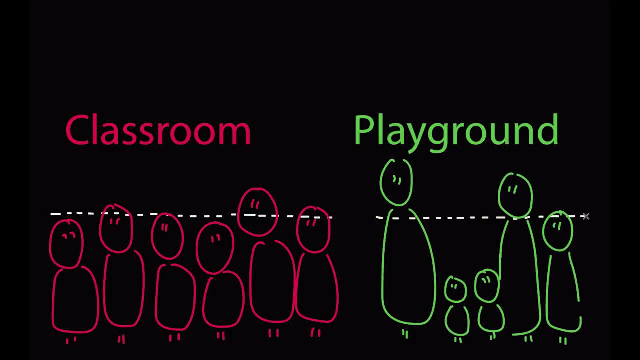 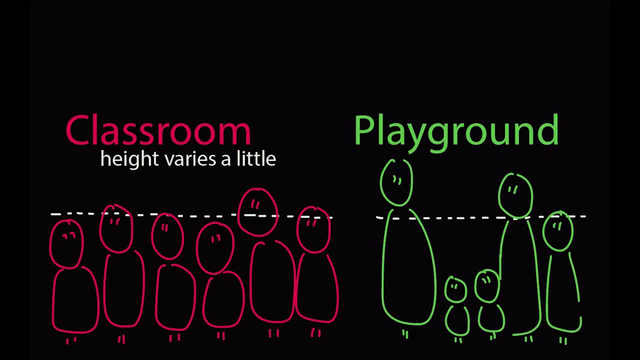 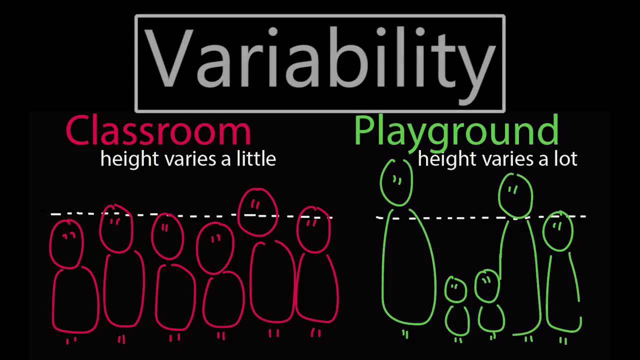 say is that height varies a little. In the playground, however, height varies a lot more. The parents are much taller than their young children, So in the playground height varies a lot. So what we're talking about here is something called variability In the classroom. 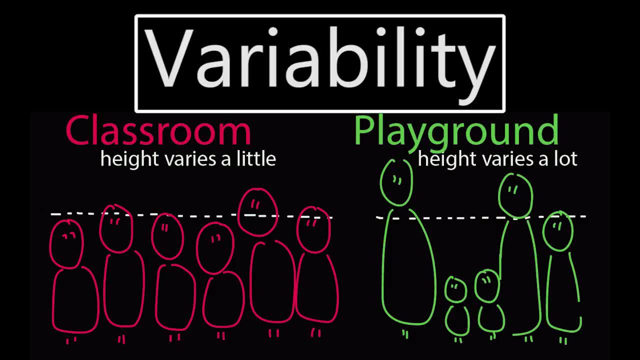 there is a little variability in height, But in the playground there is a lot of variability in height. So to go back to our question, how do the two groups differ in relation to height? Well, firstly, we have to say that the average height is the same in both groups. But what is not the same? 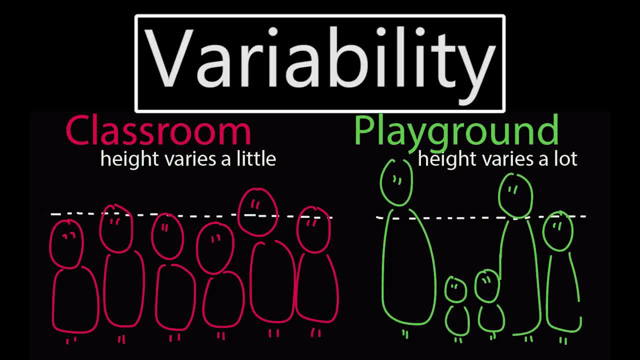 is the amount of variability in height in each of the groups. So that is why the two groups differ. They do not have the same amount of variability in height. There's a really nice way of visually representing variability. What we're going to do is draw some arrows. You start drawing the arrow at the average height. 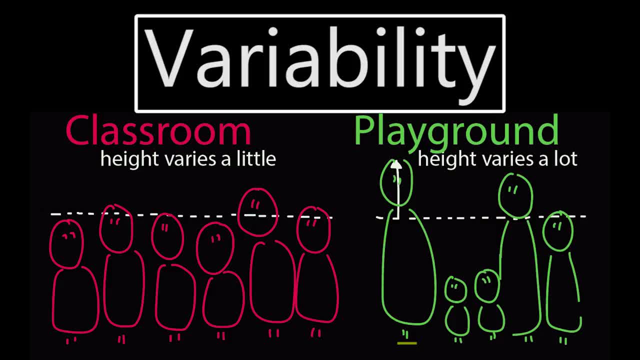 And then you end the arrow where the person's actual height is. So the babies are much below the average height, So their arrows are going to be pointing downwards. And this parent is much above the average height, So their arrow points upwards And this person 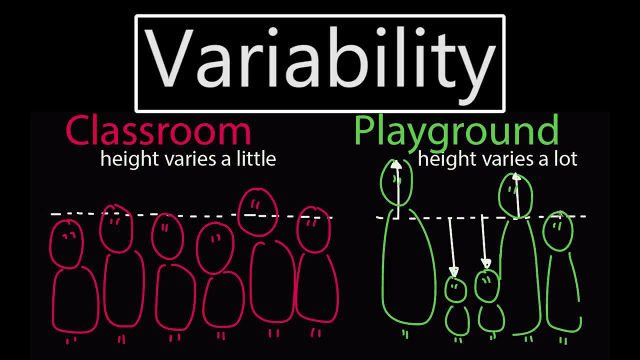 is just above the average height. Now these arrows have a name, And that name is deviations. So these arrows represent the deviations, And in this case, a deviation is the distance between somebody's actual height and the average height. Let's draw in the deviations for the people in the classroom. This person is below average height.